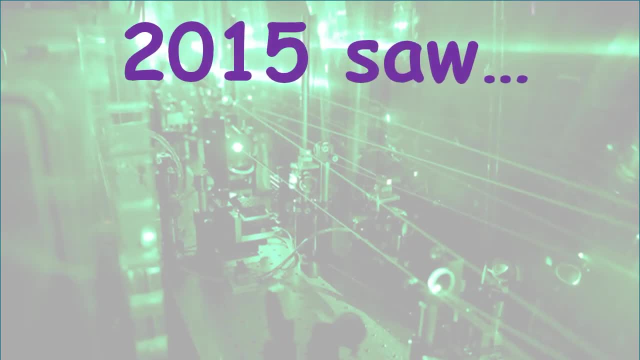 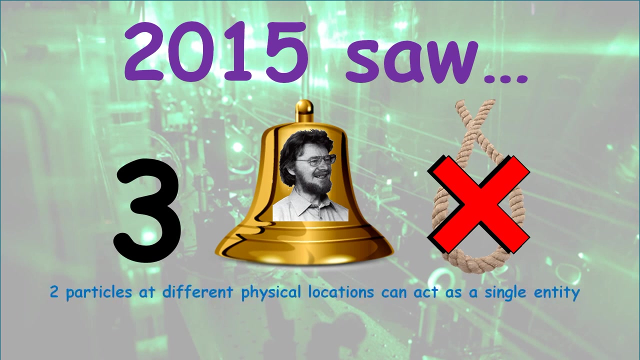 In 2015,. within the space of just three months, we got not just the first one or the first two, but the first three BELTEST experiments that claimed to contain no loopholes. These experiments appeared to show that two particles at different physical locations can act as a single entity. 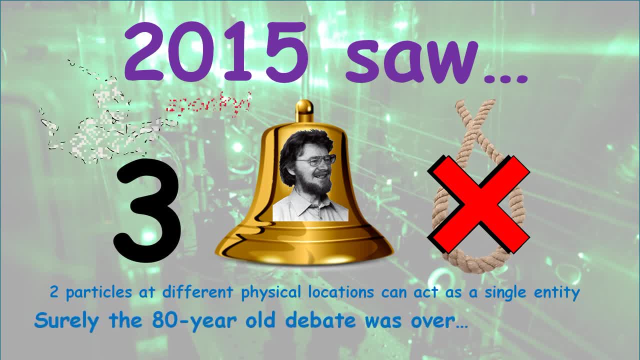 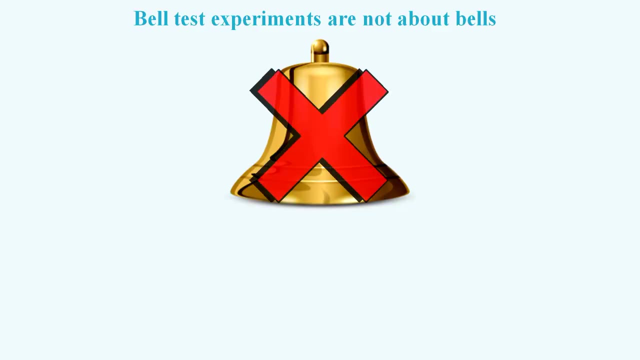 Surely now the 80-year-old debate was over. Spooky action at a distance must really be happening. Or was it just possible that there was a different and very plausible loophole that they had all missed? BELTEST experiments are not about BELs. They take their name from the physicist John Bell. 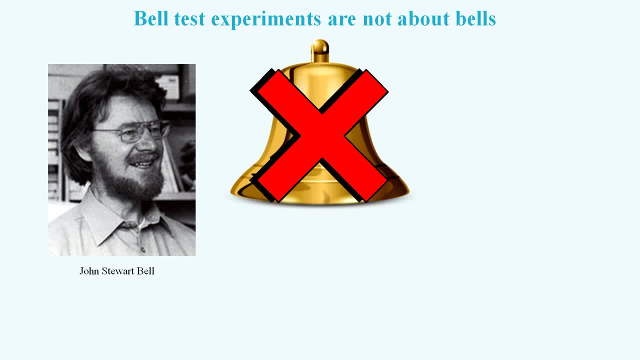 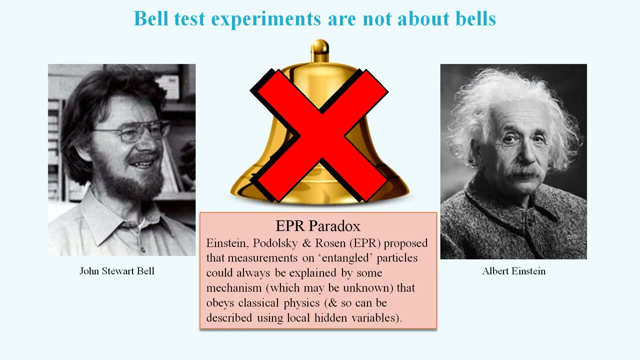 who devised a scenario for which Niels Bohr's quantum mechanics would produce different results to the thought experiment proposed by Einstein, Podolsky and Rosen. John Bell's experiment was a very interesting one. John Bell's idea can be a bit difficult to get your head around, but hopefully the following description will be relatively easy to follow. 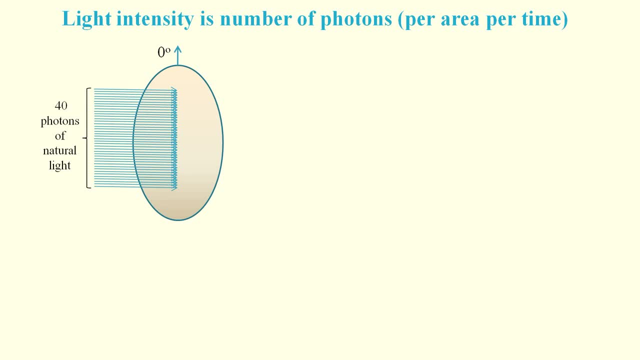 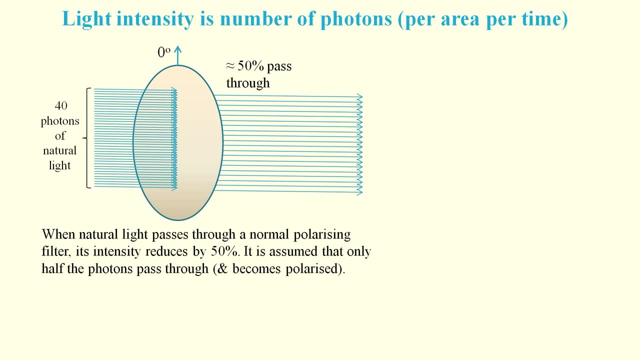 First consider natural light passing through a polarizing filter. The filter reduces the intensity of the light by 50% and the natural assumption is that only half the photons manage to pass through. If we then add a second filter where there's an angle of 20%, 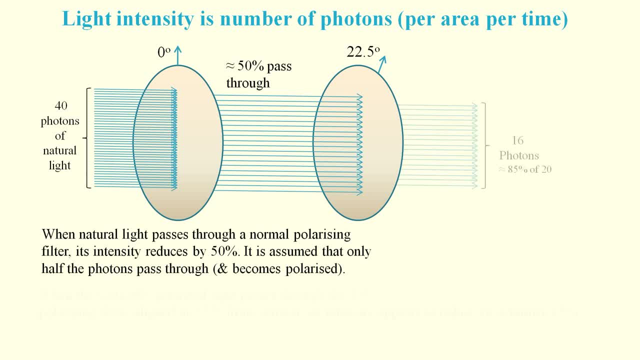 between the filter alignments, then the intensity reduces by a further 15%, And again we assume that some photons fail to pass through the second filter. From a quantum mechanics viewpoint, each photon travels as a wave of probability, and so the probability of it passing through both filters can be calculated as cosine squared of the angle between the two filters. 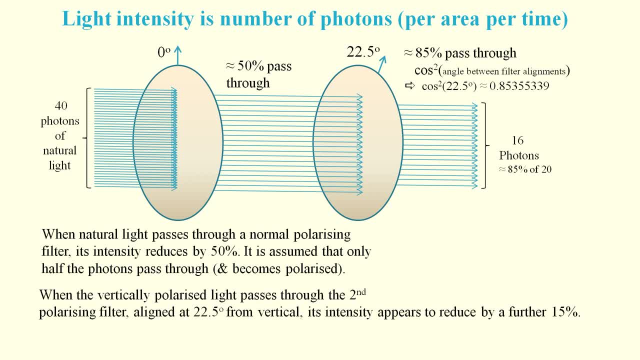 But from a classical physics viewpoint, each photon of light has its own polarization. After passing through the first filter, all the photons become vertically polarized, and then at the second filter, the intensity out is calculated as the intensity in times, the cosine of the angle between the polarization of the light and the axis of the polarizer. 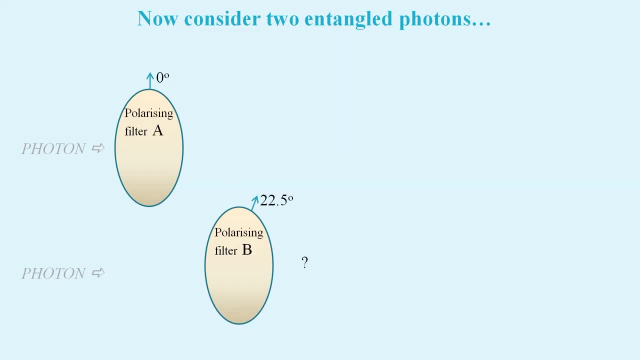 Now we separate the two filters and we send one of the entangled pair of photons through each of them. The entangled photons are supposed to act as one entity, And so if photon A passes through its filter, then by spooky action at a distance. 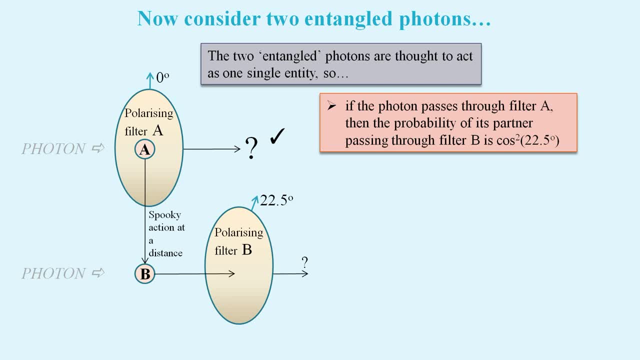 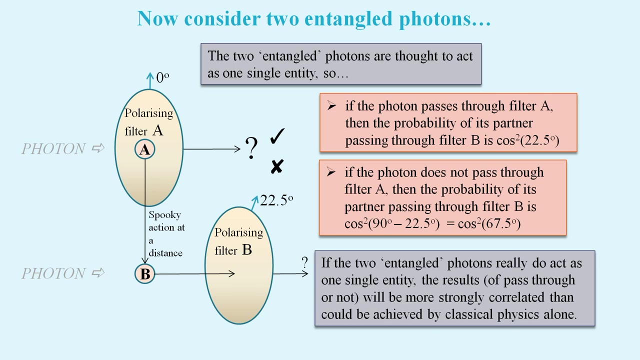 photon B will act as though it has the same polarization as photon A's filter, But if photon A fails, then photon B will act as though it has a polarization perpendicular to the alignment of photon A's filter. John Bell realized how this could be used to get results that would be impossible for classical physics to reproduce. 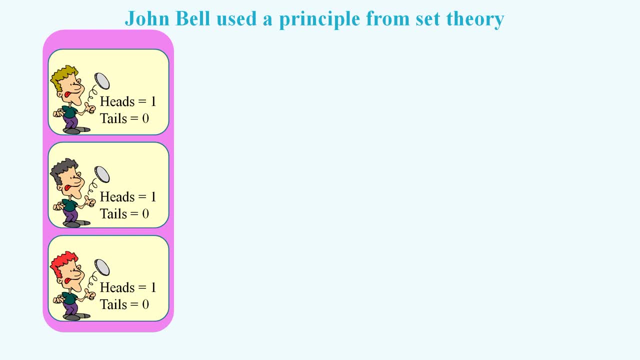 Instead of photons. consider a stream of coins being passed to three people who then flip the coins. Let's call these three people angles. The first person is a particular angle. that we'll call angle A. The second person is a slightly different angle. that we'll call angle B. 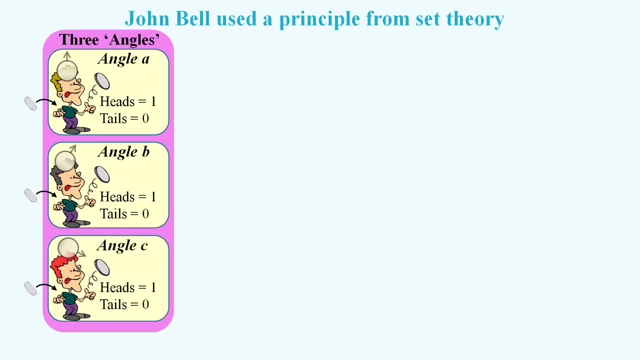 The third's another angle that we'll call angle C. Now, if all three people flip a coin at the same time, there are eight possible outcomes. Note that we denote heads as 1 and tails as 0. So 0, 0, 0 means they all flipped tails. 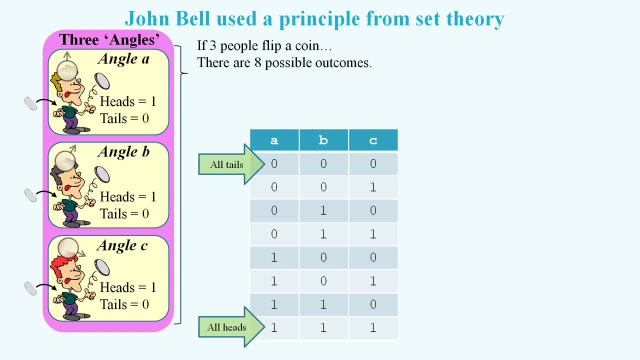 And 1, 1, 1 means they all flipped heads. If the three people keep flipping coins, then each result will always be one of these eight rows. Next we identify the rows where A flipped heads and B flipped tails, which is denoted by the column heading of A, not B. 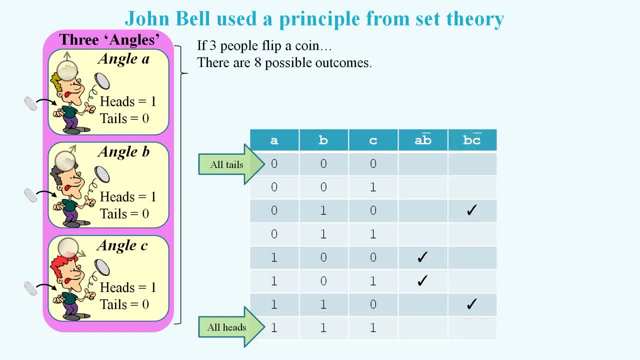 Then we identify where B flipped heads and C flipped tails And finally we identify where A flipped heads and C flipped tails. Now, if we wanted to count the number of times A flipped heads and B flipped tails, then we would need to add up the number of times these two results occurred. 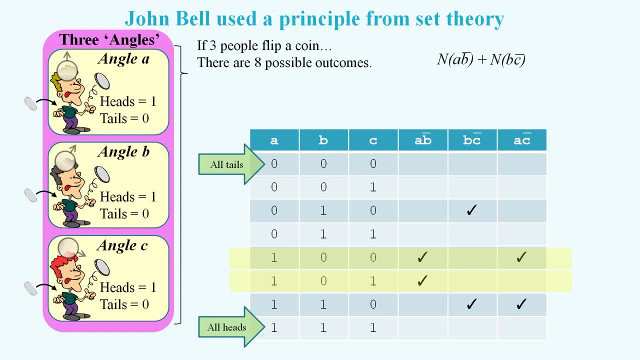 And if we wanted to add the number of times B flipped heads and C flipped tails, then we add the count for the relevant rows, giving us the count for these four rows to add up. But now consider the count for A flipped heads and C flipped tails. 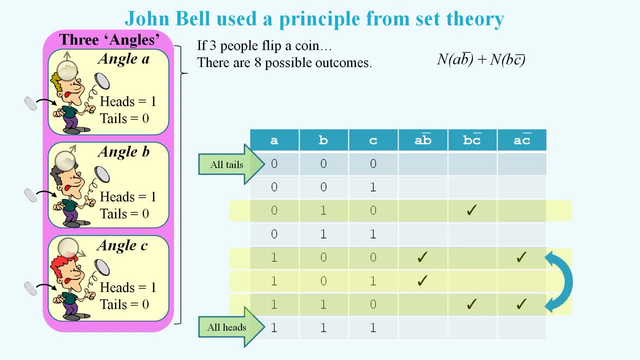 Since both the relevant rows are already part of the four rows we've already counted, we know that this count cannot exceed the count for all four rows. Mathematically, we can say that the sum of the first two counts must be greater than or equal to the third count. 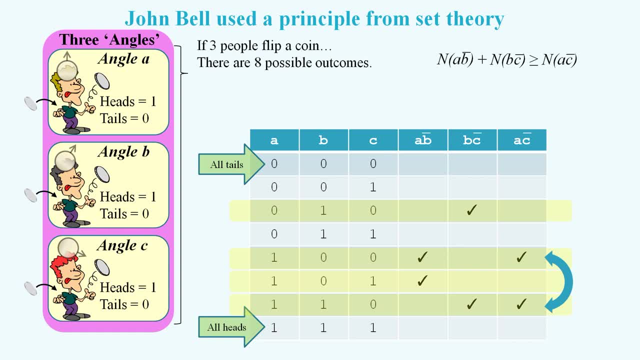 Indeed, if all three people flip at the same time, then it's impossible to violate this inequality. But what if we set up some trials where just two people flip a coin at any one time? On one side we could select between angle A and angle B. 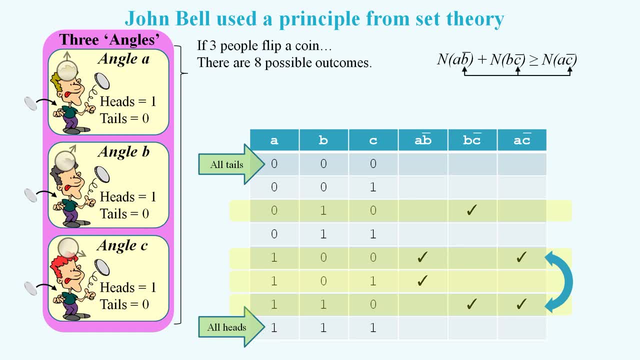 and on the other side we could select between angle B and angle C. From all the trials with angle A and angle B, we can get the number where A is heads and B is tails, And from the trials with angle B and angle C, we can get the number where B is heads and C is tails. 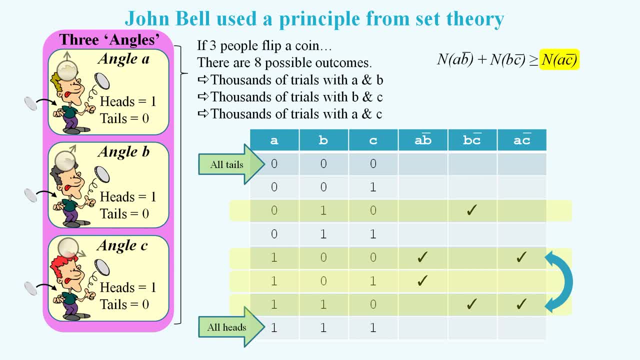 And from the trials with angle A and angle C we can get the number where A is heads and C is tails. Bell realised that if there was no spooky action going on then this should still not violate the inequality. But if spooky action was going on then it should be possible to select some angles that would cause this inequality to be violated. 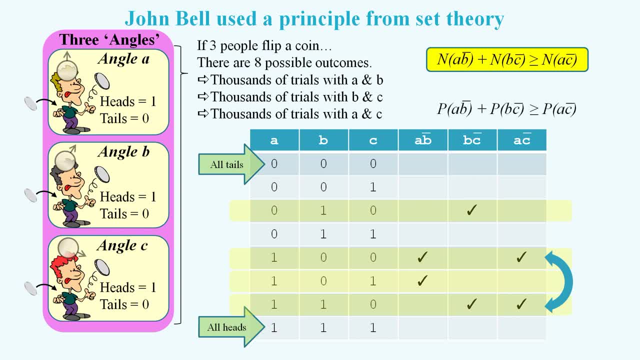 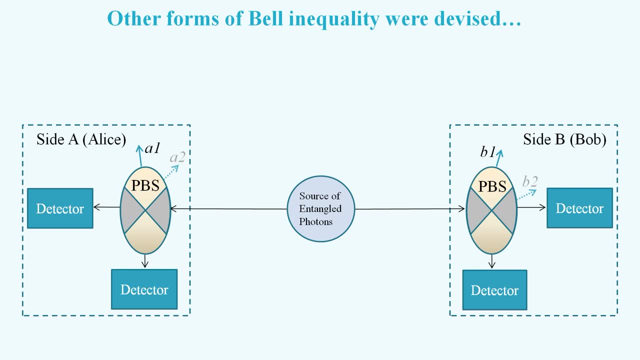 If we rewrite this inequality as probabilities instead of numbers, then this forms the original expression known as Bell's inequality. Now let's sketch out an experiment where we can select between two angles at each side. We could use a polarising beam splitter on each side so that a photon passing straight through can be thought of as heads.